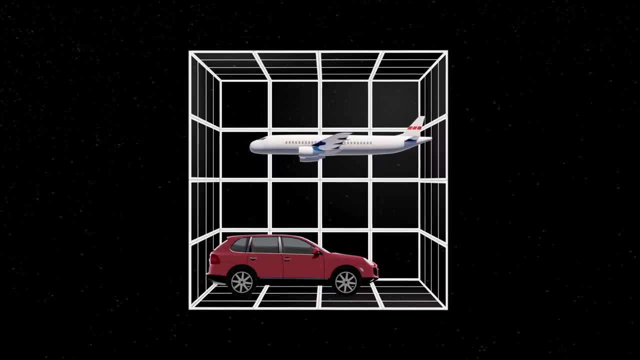 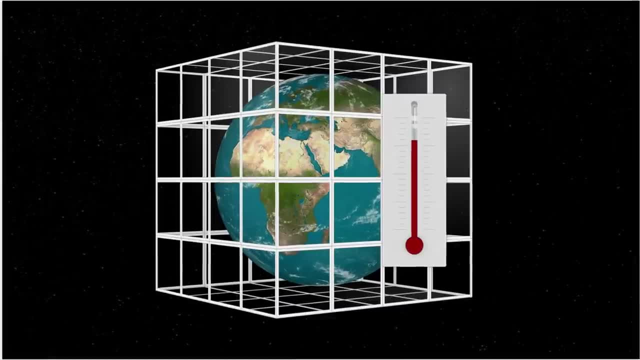 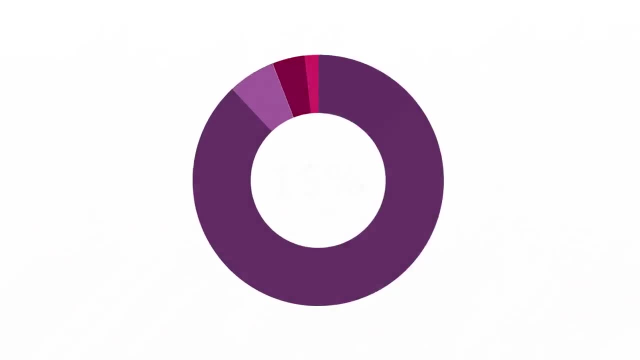 way into the atmosphere, strengthening the greenhouse effect. The additional heat is causing climate change, with the Earth literally heating up and with some huge consequences for the environment and people. Carbon dioxide has by far the greatest share of anthropogenic greenhouse gas emissions. 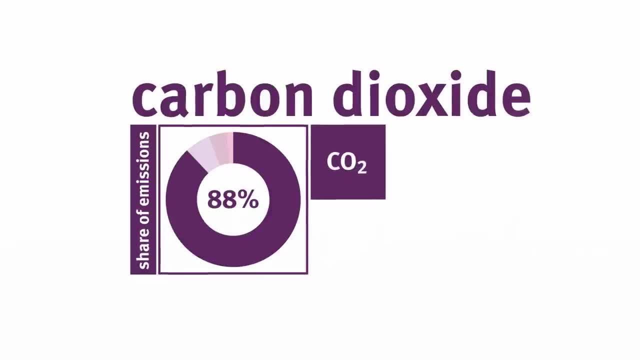 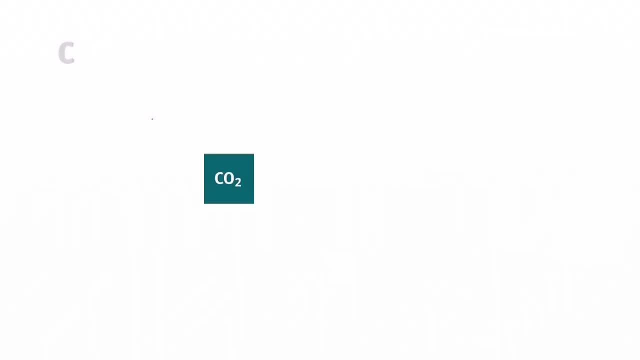 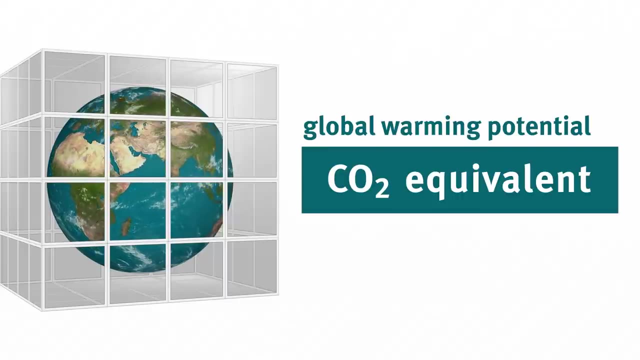 which means emissions that are caused by human activity. This mainly arises when fossil fuels such as coal, crude oil or natural gas are burned. To be able to better summarise and analyse the effects of these gases, their global warming potential can be expressed in the form of CO2 equivalents. This shows how much more an individual greenhouse gas 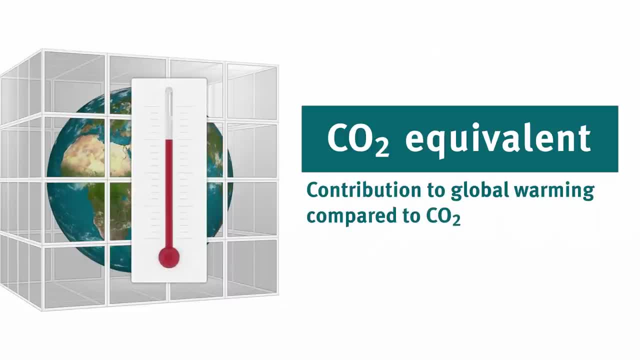 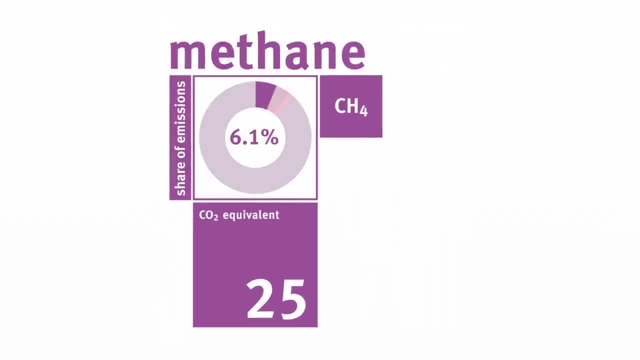 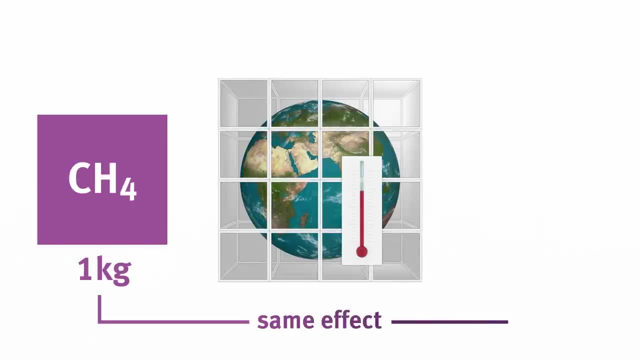 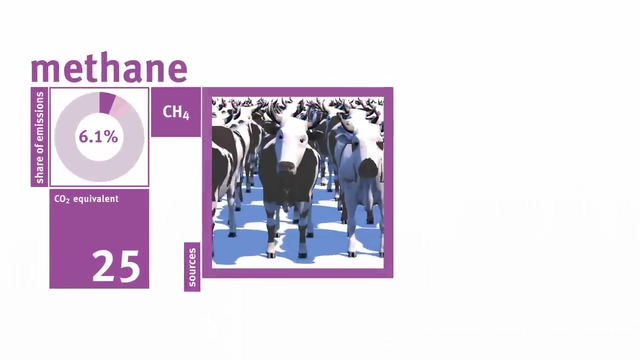 contributes to global warming in the next hundred years. Accordingly, the impact of methane is 25 times greater than CO2.. Therefore, in the first hundred years of its emission, one kilogram of methane contributes 25 times more to the greenhouse effect than one kilogram of CO2.. In Germany, methane largely arises through 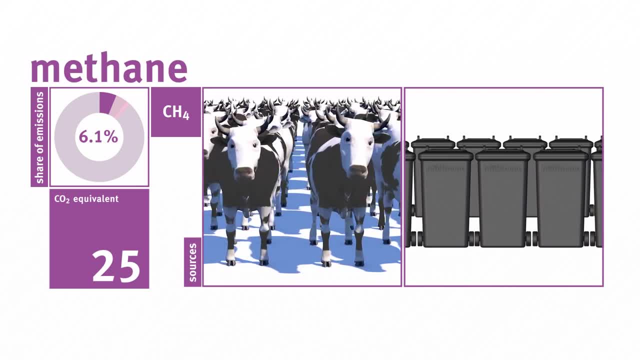 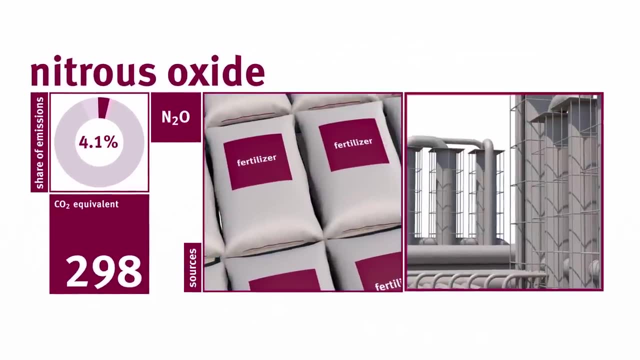 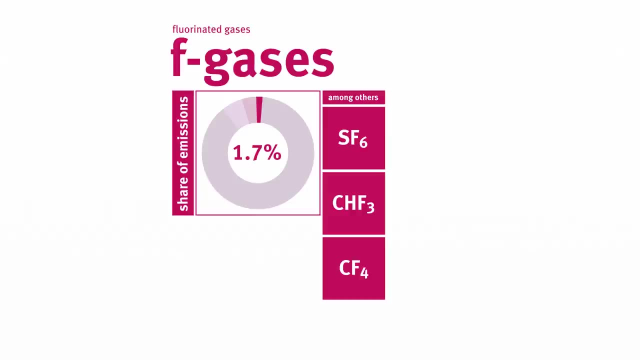 agricultural livestock farming and the waste sector. The impact of nitrous oxide is 298 times greater than CO2.. This mainly arises during the production and use of fertilisers and in the chemical industry, Although fluorinated gases only account for a very small proportion of total emissions. 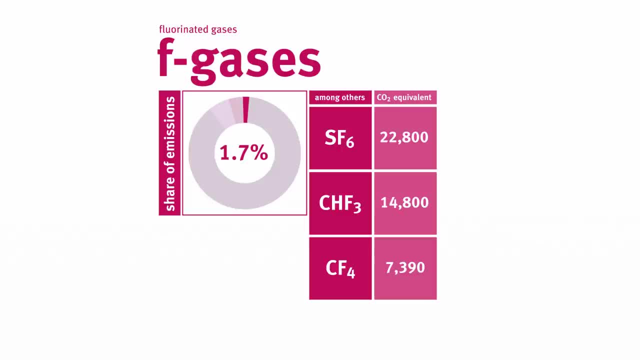 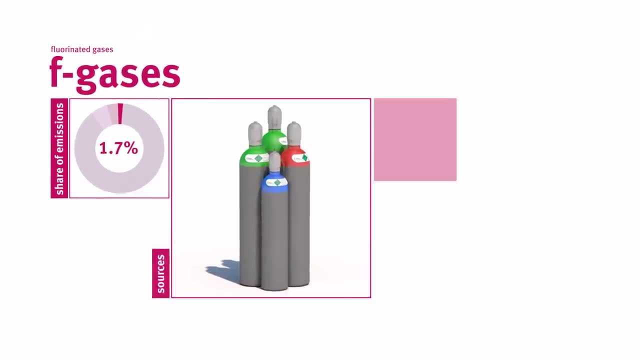 some of them have an extremely potent greenhouse impact. The CO2 equivalent of sulphur hexafluoride, for example, is 22,800.. F gases are used as coolants and extinguishing agents, as propellants and insolvents, among others. 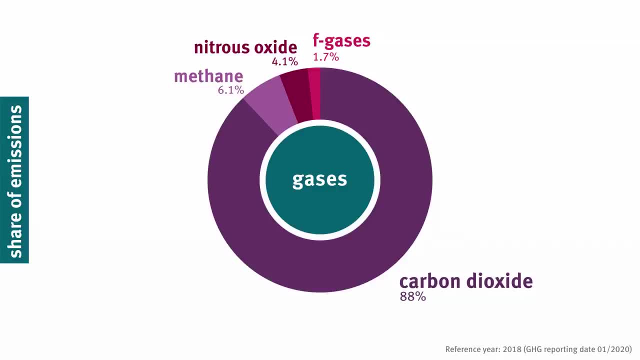 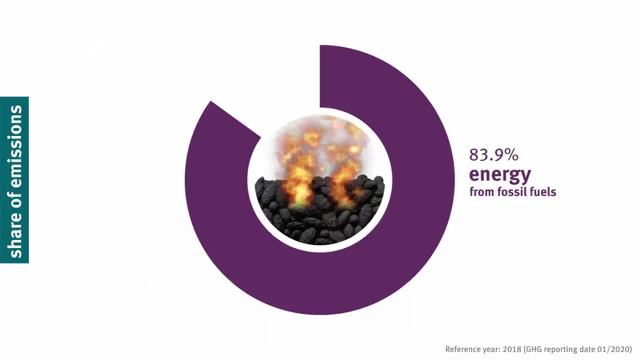 In Germany, most greenhouse gases are produced by the greenhouse. In Germany, most greenhouse gas emissions arise when fossil fuels such as oil or coal are burned to generate energy. The primary source in this area is the energy industry, for example, the generation of electrical 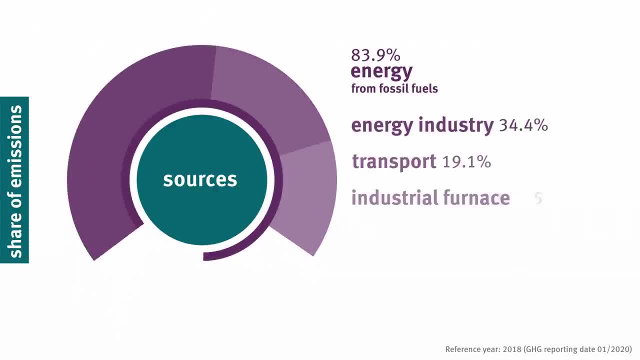 power and heat. This is followed by transport, industrial furnaces, private households and the commercial, retail and service sectors. Other emissions are caused by the production processes in industry, agriculture and waste management. If emissions from energy production are limited, there is a risk of a global warming. 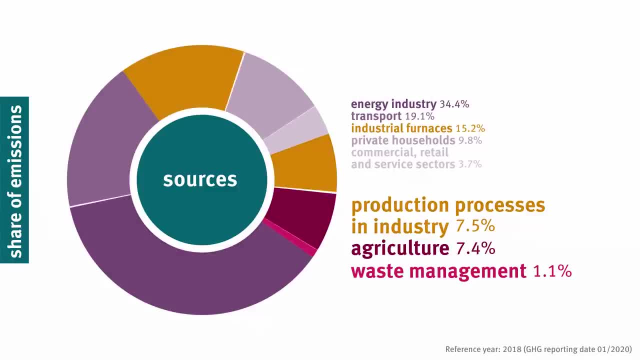 If emissions from energy production are limited, there is a risk of a global warming. If emissions from energy production are limited, there is a risk of a global warming If emissions from energy production are broken down and the share accounted for by industrial furnaces.